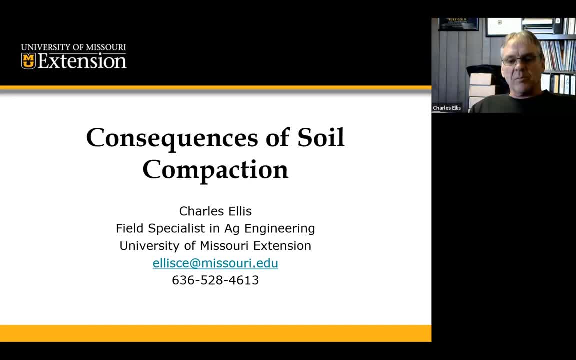 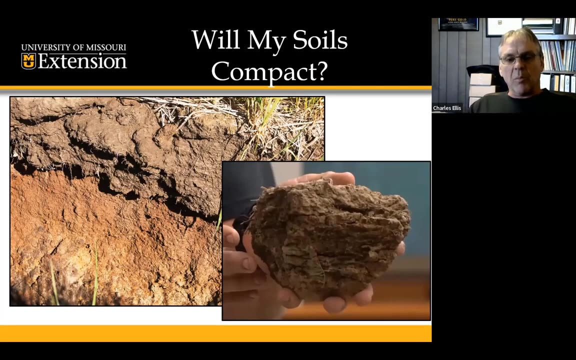 I hope to join you for the question and answer session of the webinar, so hopefully this will work out. So, when we talk about soil compaction, when we're working with producers in Extension, when they have questions about crop production, they want answers of. when I make a change, will it make a change in my production practices? 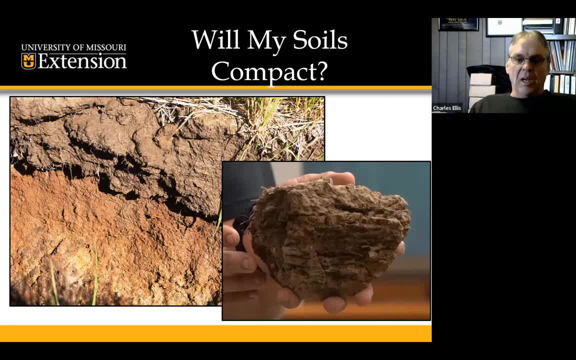 So they're looking for changes that will change in yield and you know an example of that would be adding irrigation to a crop field will get an increase in yield. But when we get to an issue like soil compaction and they ask, well, what the effect is of that, then we get in that area of you know mites and maybes, I guess we call it. 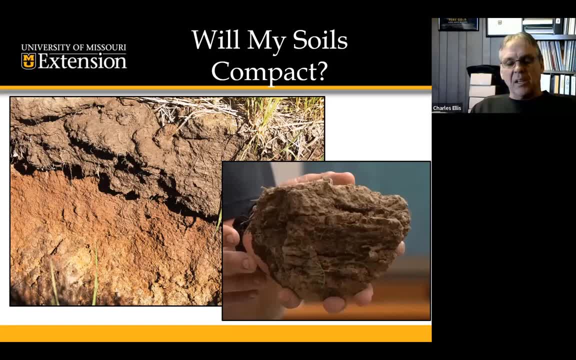 and we have a lot of that in production ag and it can be a frustration- Producers and you know, and Extension people as well as trying to determine what is happening out there in the world, And you know we have to take that data that we have available and make the best judgment call for our operation. 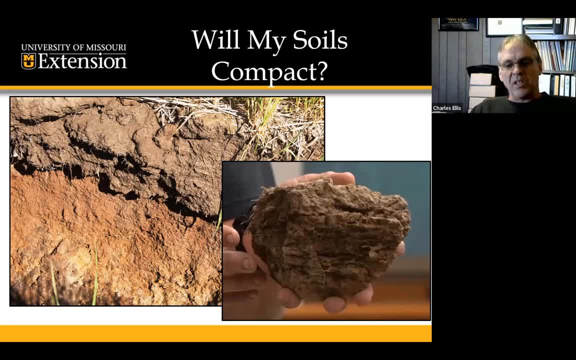 And ultimately it's up to the producer to make that call on their operation. So I want to talk about, you know, the soils. will they compact? And they will. This is soils for in my part of Missouri and they have a high clay content. 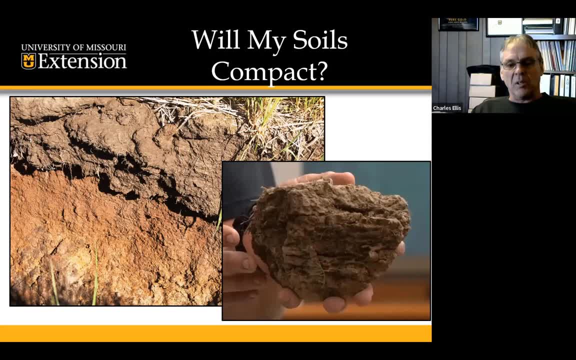 And in this area of the state many of the small towns used to have brick plants. So you know, with that soil type and profile they were, they are susceptible to compaction, as you can see in that picture in the right. 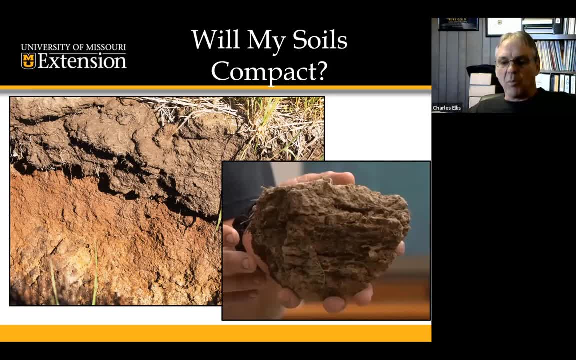 where we've got a lot of horizontal stratification from, you know, wheel traffic causing. that's not where the soil compaction occurs. So we do have soil compaction. that will happen when we get into the mites and mavies is what 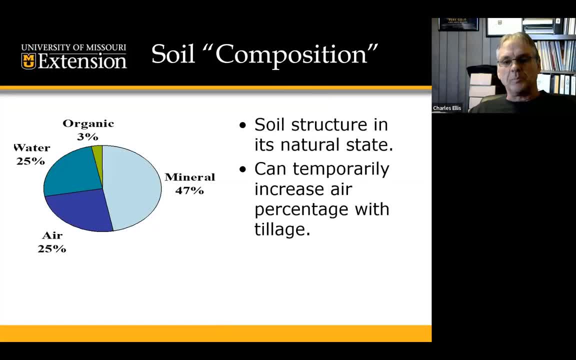 what is the outcome, you know, from that soil compaction. So when we look at the soil composition, we can look at it in its natural state. It's going to be typically about 43% mineral, with about 25% air and 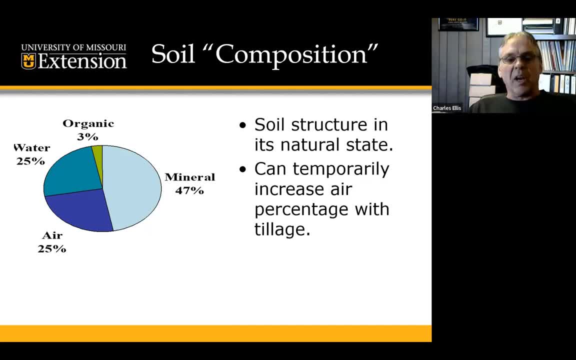 and 25% soil compost water with about three percent organic matter. for my part of the country, Missouri, soils will be in that area. depending on the location you're living in or picking the webinar from. You're going to vary from that, likely higher or lower from that and some things you know we can temporarily. 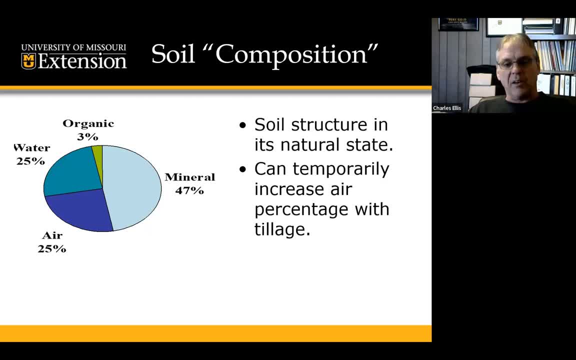 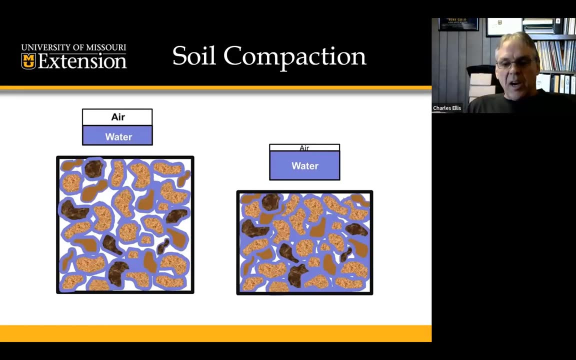 increase that percentage out, you know, with tillage doing that artificial fluffing of soil. But over time it's going to kind of come back to that equilibrium that I'm showing there in that pie chart. Schematic here of soil compaction is when we run wheel traffic or have a tillage. 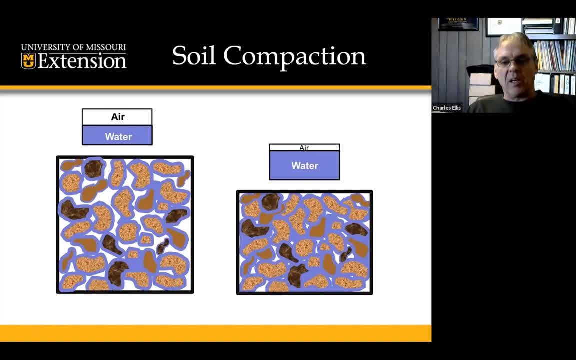 implement run in wet conditions. We are compressing that pour and water space down. I mean we're pushing that those soil particles there closer together. We're removing that poor area there that's either going to limit air or water from being in that soil profile. Here's another. you know this this. 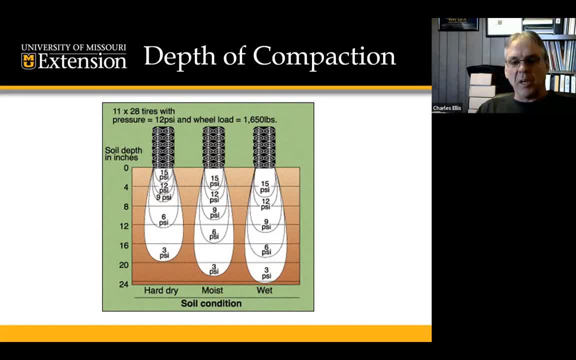 will happen. It's not a might or maybe, when we come, when we run over soil with our, with our tires, we're going to have a compaction going down into that soil profile. Granted, it may be minimal or to the or to an extreme, depending on factors such as soil conditions at the time. 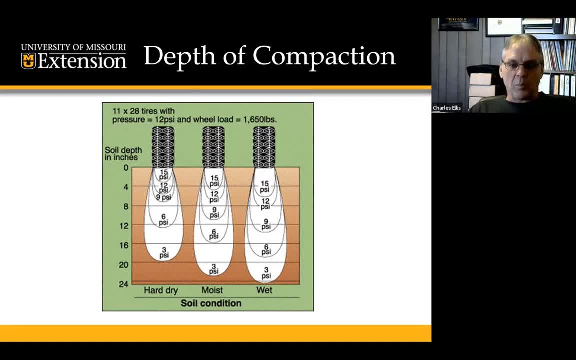 soil, moisture. size of tire. size of footprint of the tire, weight on the tire. weight of the axle. This is just. I don't mean for you to take an absolute number from this graph, but just showing the differences you'll have transitioning from a dry to a wet soil, How we get that. 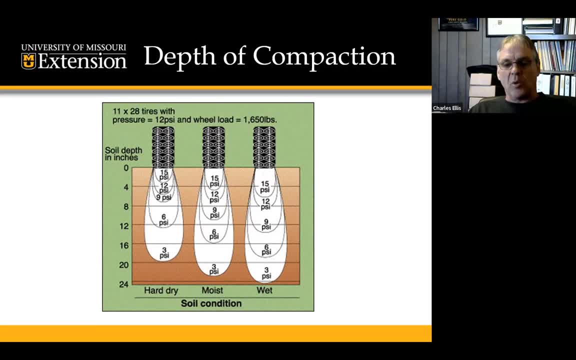 pressure or compaction to drive down into that soil profile. as we go from a drier to a wetter soil You can see we can real quickly get past what tillage implements are capable of getting to if we're trying to remove compaction to the soil. 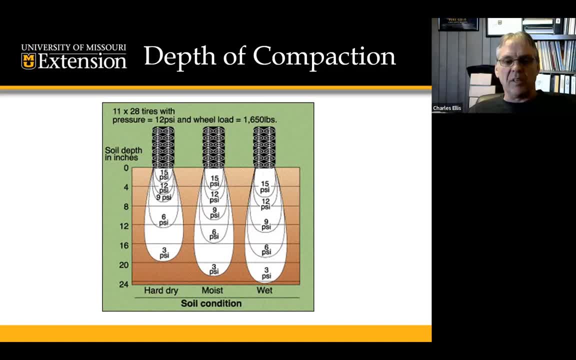 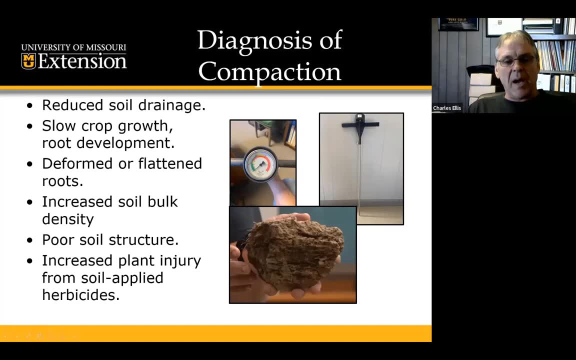 Compacted layers with tillage that's been driven deeply into the soil profile. When we're trying to diagnose if we do have compaction in the field, there's a lot of visual observations we can. we can see out there: Reduced soil drainage in the soil profile, Slow, you know crop growth and root development. you know which would we. 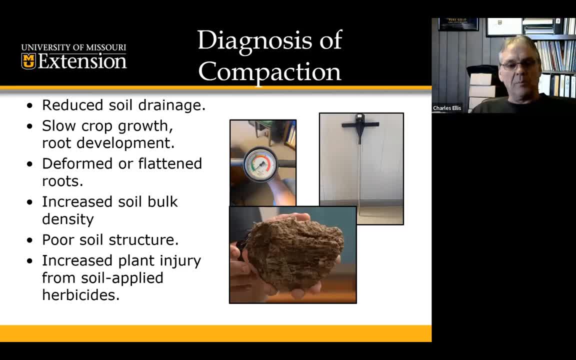 be related to deformed or flattened roots growing there. in the soil Measurement of soil bulk density- increased bulk density occurring, you know poor general soil structure- We could start to have some increased plant injury from soil applied herbicides show up. you know, due to these changes in the soil profile. If we're going to try to measure, 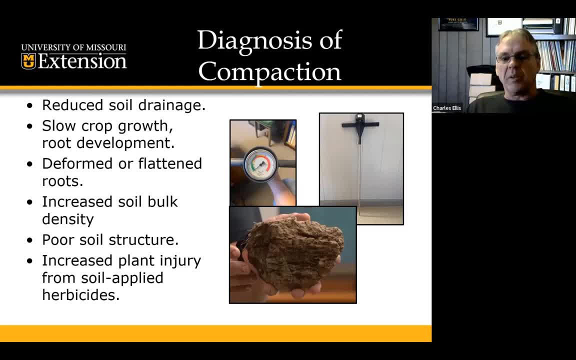 soil compaction. one method would be with the penetrometer. This would have a dial on the instrument. We would push that into the soil profile and what we're looking at during that time is looking at the reading on the dial as we're going through the soil profile to try to determine. 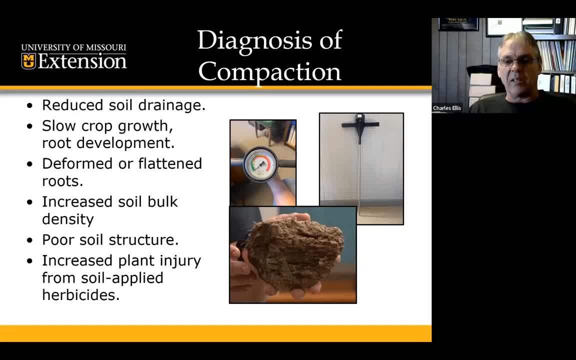 if we have have and where we have compacted layers in that profile And what we can use this far is is determine where the compacted layer may be at And also maybe also see in a field where the targeted compacted layers may be, you know, in the field, whether it be field. roads turn roads. 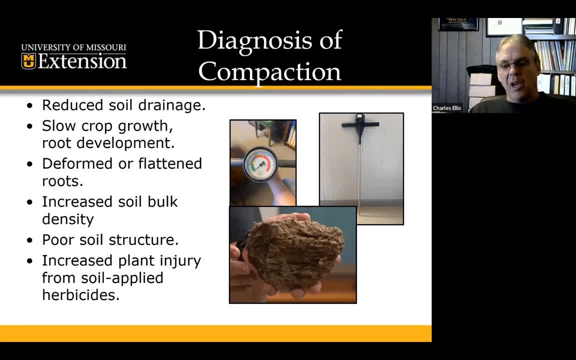 field borders areas like that. It's not intended to make a absolute number or value out there because you know soil conditions that day are going to determine or influence those, those numbers on that reading. You know what, what the readings you're going to get in April are going to vary from what you might get in August in that same location. 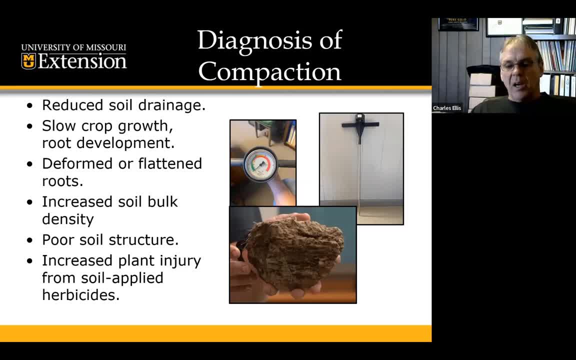 Another method would just be, you know, digging up soil samples or pieces of soil and looking at their soil structure, how they're changed in different locations. With this photo on the bottom, with you know, the horizontal plate structure we have there, you know, showing some compaction from a from a field road. 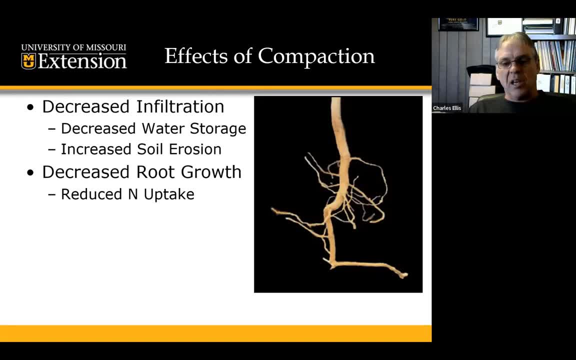 Roots or plants in roots can really tell us a lot. When we start getting into a lot of compaction issues we get diminished root growth And with that, know we start getting some of these other issues. But you know the the compaction also. 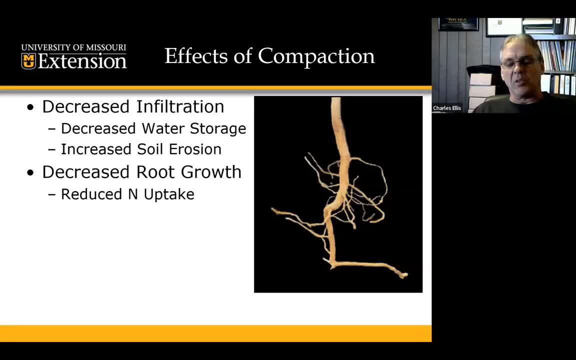 leads to decreased infiltration into the soil and becoming more root, so it's a good way to keep the soil covered. cause of that, we're not getting as much water into the soil- decreased water storage in that soil profile because we compacted, pushed that, limiting that pore space that we originally had. 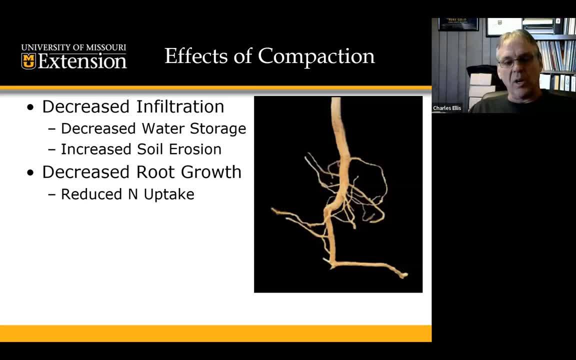 Less water is entering the soil profile, so we have more surface runoff, which has potential to increase soil erosion. due to the diminished root growth there, We're going to also experience reduced nutrient uptake, particularly nitrogen. We can start seeing some stress even where we have 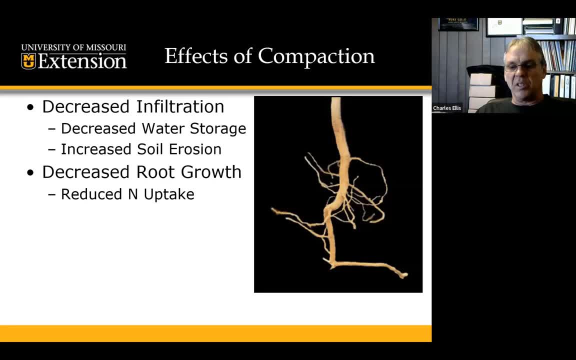 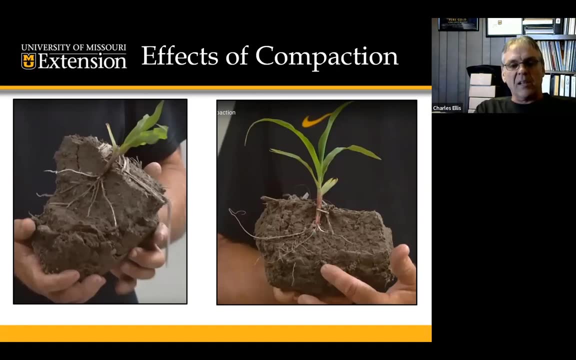 soil test readings showing sufficient nutrient levels out there. Just the fact that the plumbing from the roots are not sufficient out there. These are photos I took. this is compacted root zones in a corn crop, calledutable, caused by the planter being planted in wet conditions. 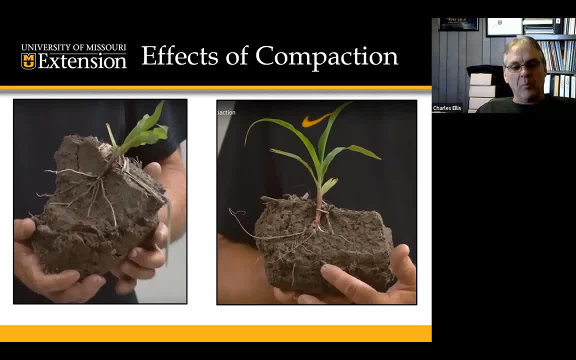 not necessarily by wheel track, but you can see how the root development's been inhibited by the compacted seed slot. there We've really just got root structure going in two directions in the seed slot, horizontal roots being developed And you can see over time with lack of root development. 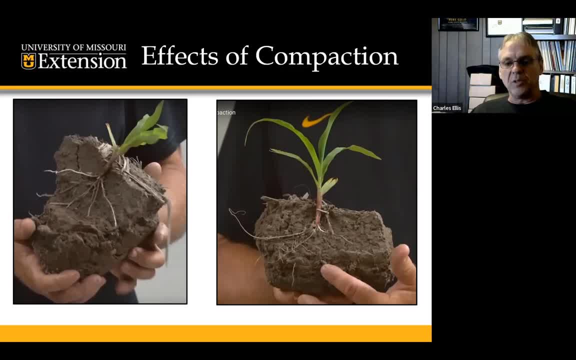 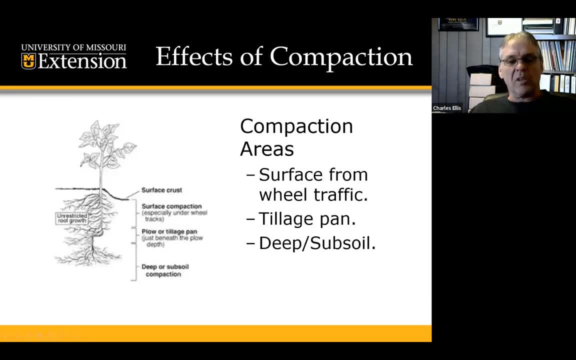 we're going to start to have a lot of nutrient deficiencies and poor growth from that corn plant. We want to look at a profile of a plant here to help kind of diagnose the areas we could have compaction. We can even have surface crusting. 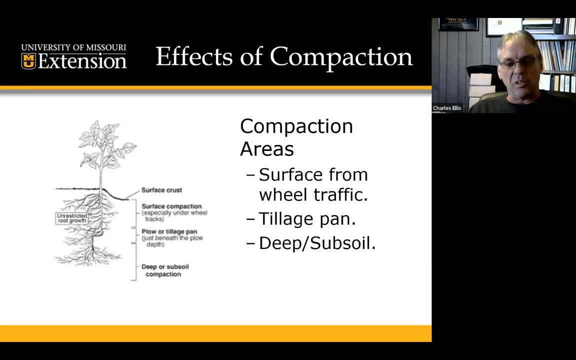 You know, if we've got finely tilled or some soils that are susceptible to crusting just from rainfall events, we can have just wheel traffic going over some tilled soils. We can have root development a little bit further down from historical tillage or plow pans. 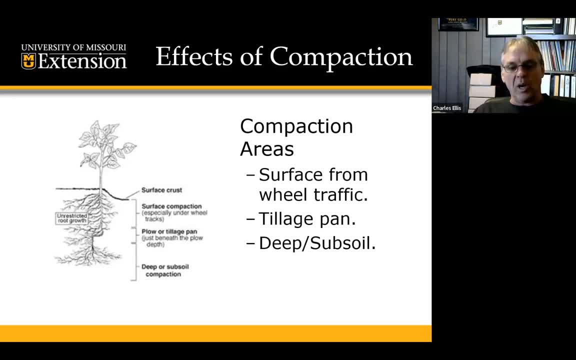 that developed years ago. looking at long-term management of the field, We might still have some of those issues And then also we might, digging the roots, find some deeper or subsoil compaction that may be from natural soil, compacted areas or subsoil properties. 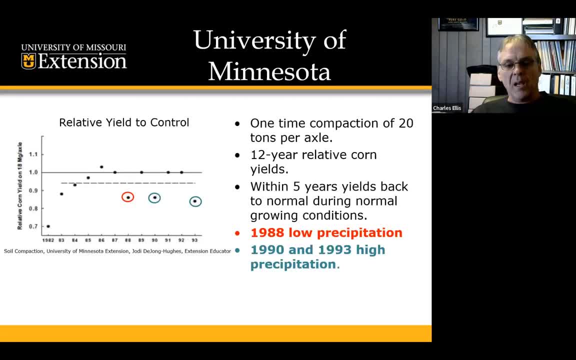 that are in our soils. Now I'm going to get into kind of the mites and maybes of soil compaction. This is where you know producers would like to know the. you know the absolutes, but when we start talking about yield from soil compaction, 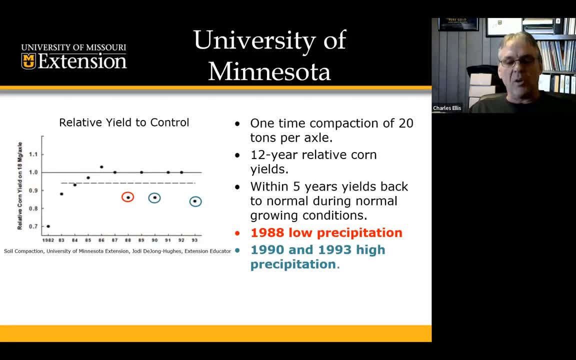 this is from a University of Missouri Minnesota publication where they did a one-time compaction. you know soil compaction. You know 20 tons per axle And it's looking at 12 years of relative corn yield. So they didn't do any. you know tillage. 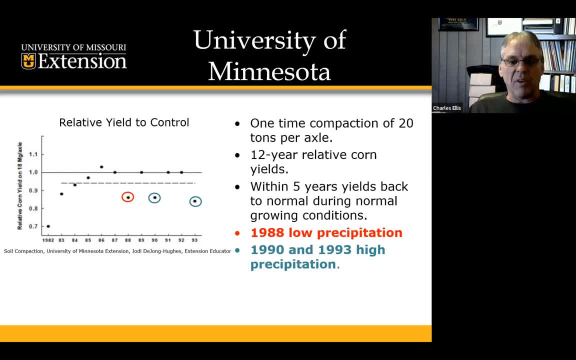 to try to mitigate the compaction And within five years, you know, the soils had rebounded on their own back to normal growing conditions. But when we had in that 12 year period they also had you know three years, what they called. 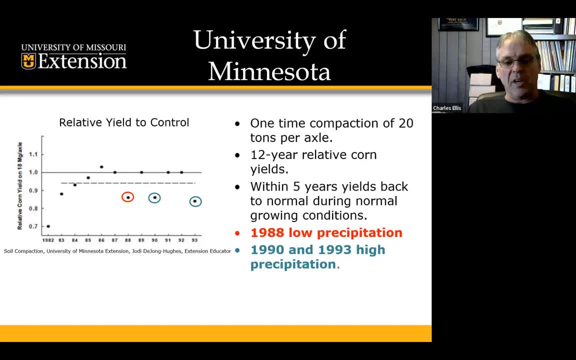 you know, I guess, stressful growing conditions of one, two, one year in red of low precipitation, in two years there in the blue above normal precipitation, And in those years where they had the more stressful growing conditions the compaction event still shows up. 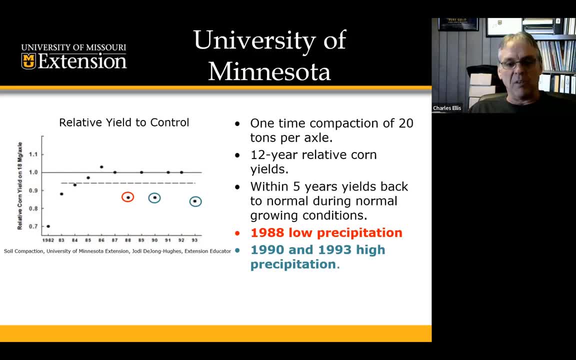 as a reduction in yield. you know down, you know 10 to 15% reduction in yield. So it's kind of where I was coming from. you know on the, you know good growing conditions can mask a lot of. 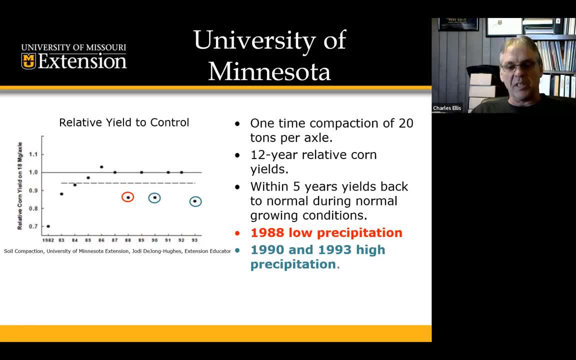 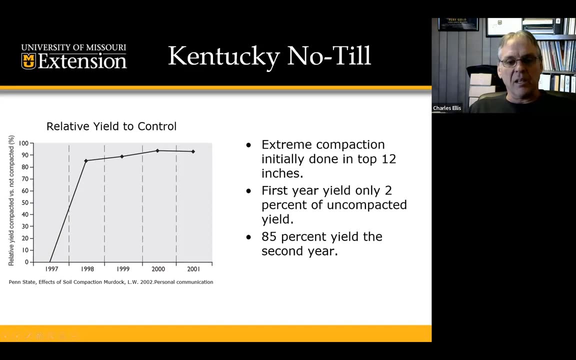 you know other effects or other limitations And when we start getting into these more fringe growing years some of these problems will start to crop up. Another study in Kentucky, in no-till, where they did a lot. you know extreme compaction. 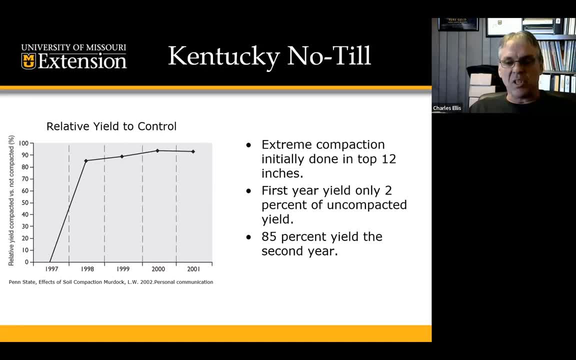 that's how they defined it. in the top foot They were seeing only- you know- minimal yield. It came across. what you're seeing is lower, you know wird. So what- the idea is that you might see moreым minimal yield that first year of 2% yield that first year. 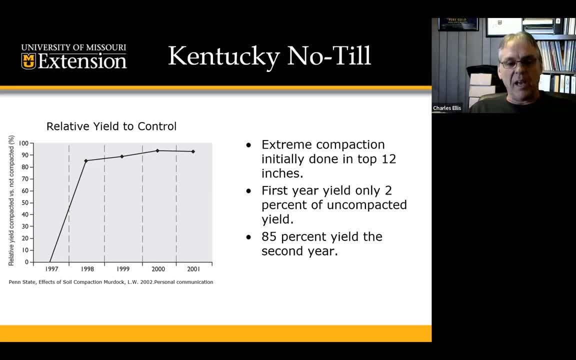 And then the soil had rebounded to 85% yield that second year still out. four to five years later they weren't back to the 100% yield. but this is also showing that the soils do have some capacity to repair themselves and rebound. 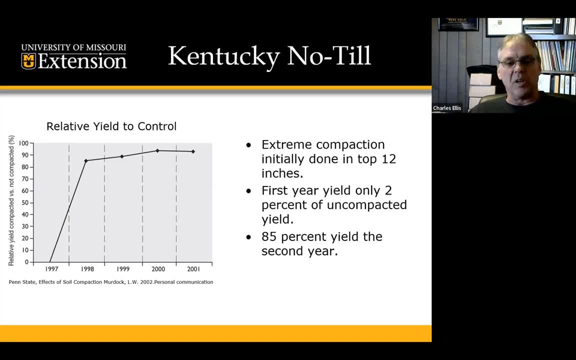 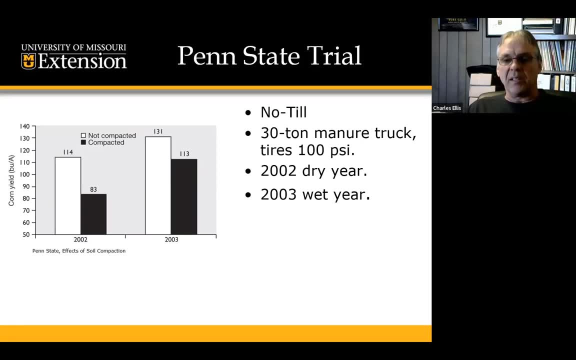 You know, on their own, without you know the tillage strip happening And then kind of back to the you know might and maybe a scenario of effective yield from soil compaction. you know Penn State trials in two years again. 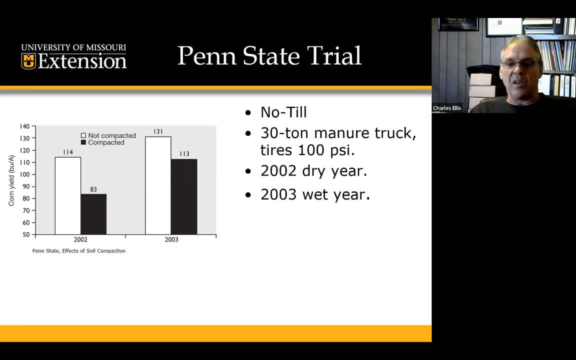 with some of those more stressful growing conditions under no-till, where the soil is compacted. you know, with the 30 ton tires. you know, in 2012, what they defined as a dry year. they had a significant yield reduction there from 114. 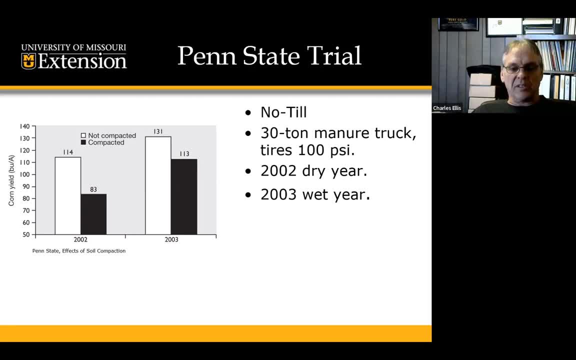 down to 83 bushels per acre And then in 2003,, as they defined as a wet year, they had a you know reduction there from 131 down to 113.. So again, in those you know years where we don't have those, 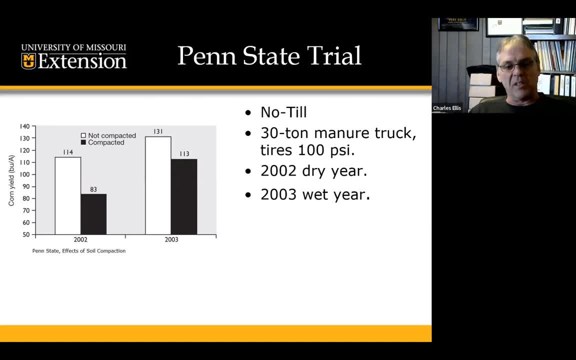 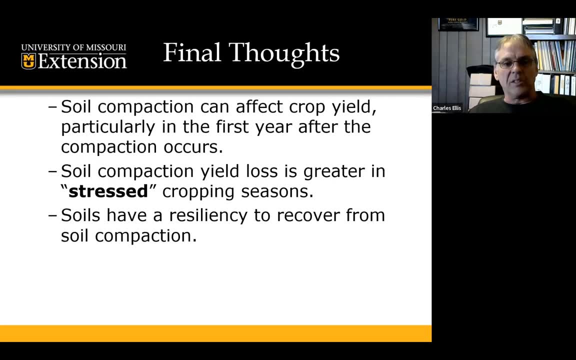 perfect growing conditions, then we're seeing the soil compaction events kind of being accentuated in those years. I'll leave you some final thoughts here. Soil compaction, you know again, is going to affect crop yield, particularly in that first year after compaction occurs. 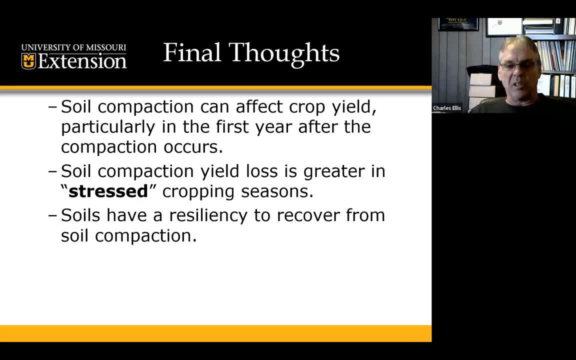 And then it can also affect you in those succeeding years where you may have a stress: cropping seasons, where they'd be wetter growing or even dry growing seasons, But the soils also are, you know, in some of these studies will show a real resiliency. 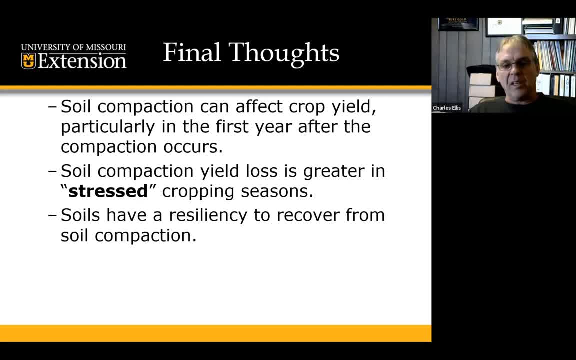 to recover from soil compaction on their own. So again, you know I'm kind of leaving you with. you know, consequences of soil compaction. Yes, it does happen, but we do kind of have some of those mites and maybes from soil compaction, of